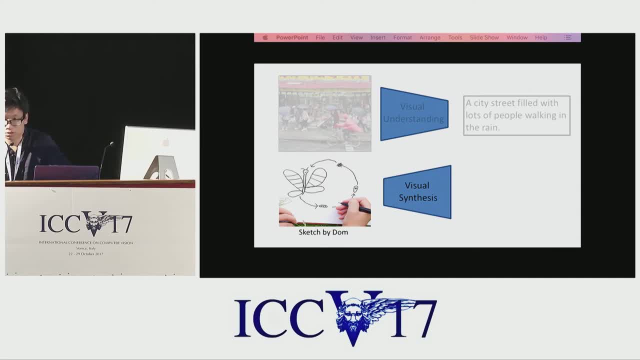 did similar things. So fortunately, his father, a Photoshop artist, turned his son's wild imagination into the realistic renderings. But not many of us are creators or have a father with Photoshop expertise. So in this talk we aim to build machines capable of generating and manipulating. 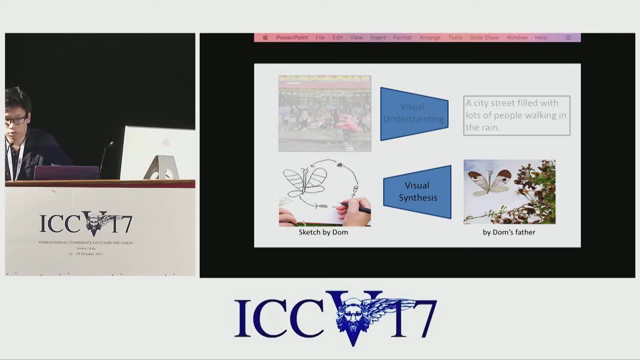 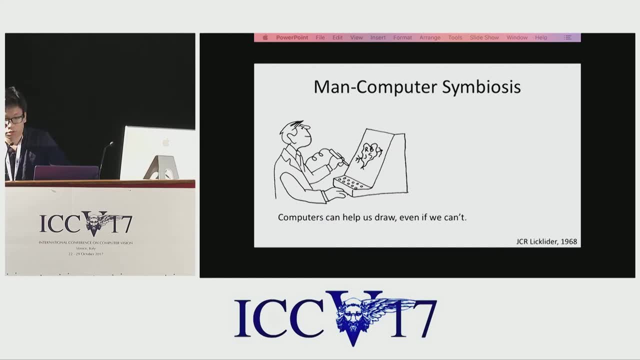 photos and hopefully can use it as a training tool. So we are not the first one to look at this direction. So the cartoon above is from a seminar paper written by J C Alec Leiter from MIT, So already in 1968,. 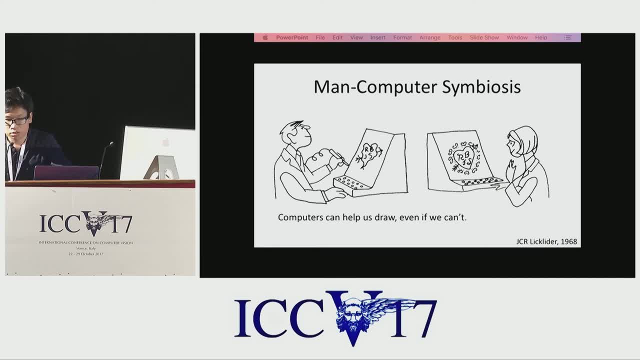 he imagined that we can build a machine to help us communicate our ideas in pictures, even when we're not good at it. So here is a picture of heart. Maybe you can enjoy it, but maybe the machine can help you generate a better heart or love images, And also along the 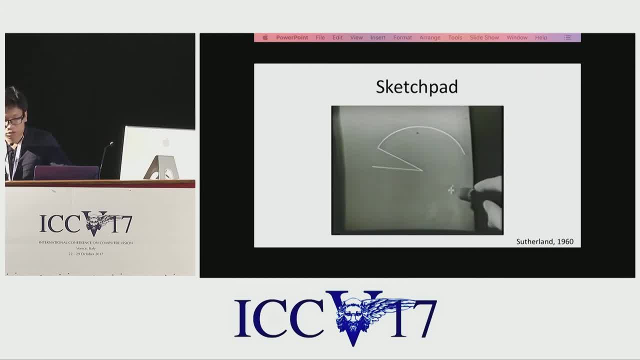 same line of sight we can create a picture of a heart. So here is a picture of a heart. Maybe you can enjoy it. but maybe the machine can help you generate a better heart or love images. And also the sketch pad project by Sir Seth Lent proposed a human machine interface where a computer can turn. 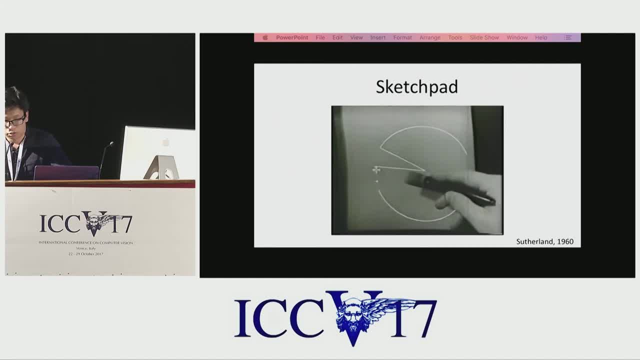 users' intent into very simple drawings. So, but even after decades of research, with the latest and best software, it's even very hard for regular people to manipulate photos. So here we show a demo of changing the shape of a handbag. So I think there are why it doesn't work. There are 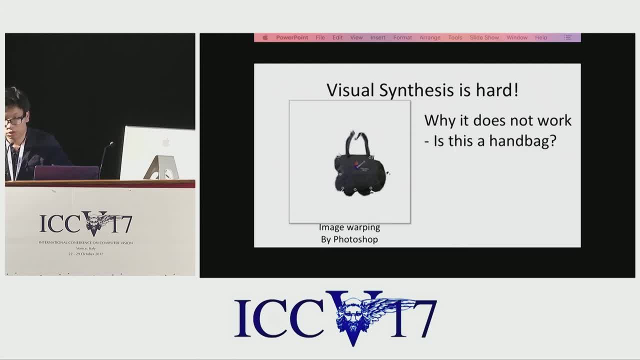 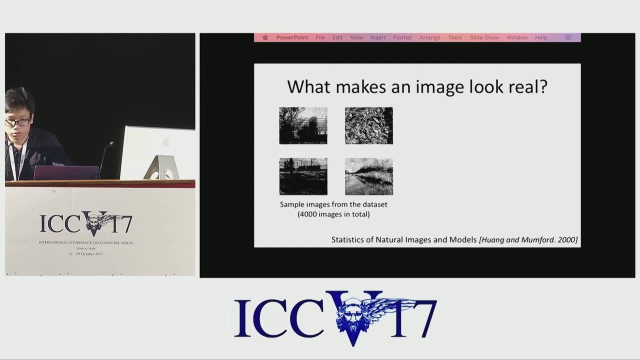 probably two reasons. First, the algorithm doesn't know if I'm editing a handbag or editing a shoe. also, the algorithm doesn't know what makes a real shoe look like real. So what makes the image look real is one of the most long-standing problems in computer vision, So back to 2000,. 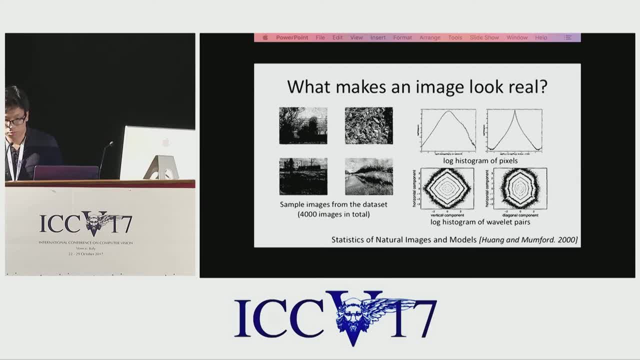 Huang and Moffat looked at some simple statistics of pixels like histogram or features like wavelets, and they can fit. they can. they can compute a histogram over the training set and you have a test set. If you don't fit this histogram, it might be fake. And also the graphics researchers. 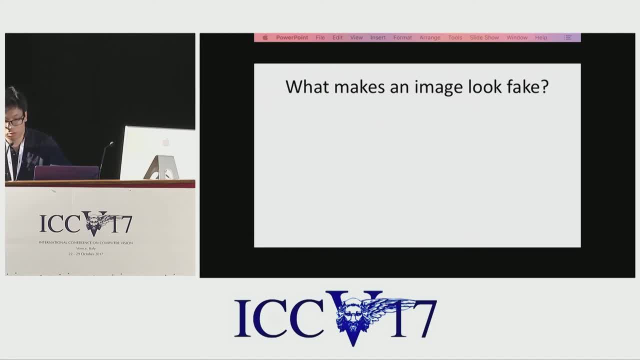 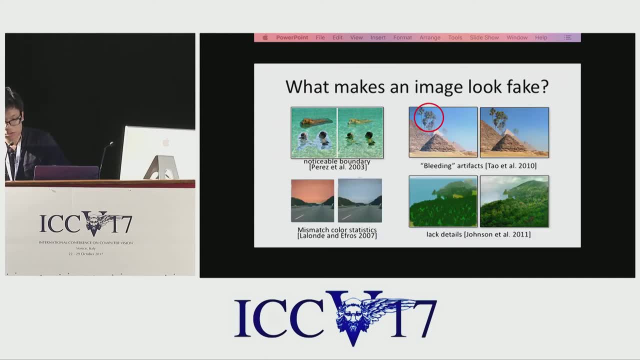 look at the problem in a different angle. So they will ask: what makes the image look fake? So people are looking at low-level cues like boundaries, color inconsistency, maybe there are no texture in the images and the manually designed individual algorithm to improve the realism of the 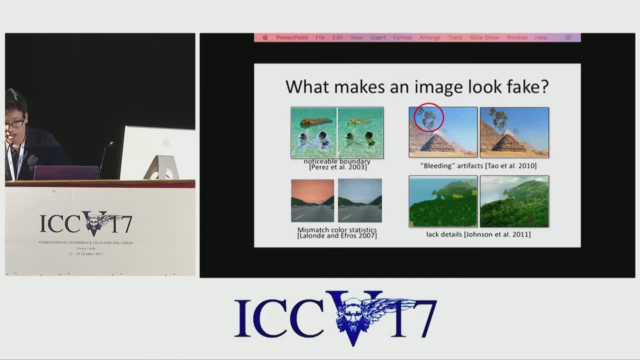 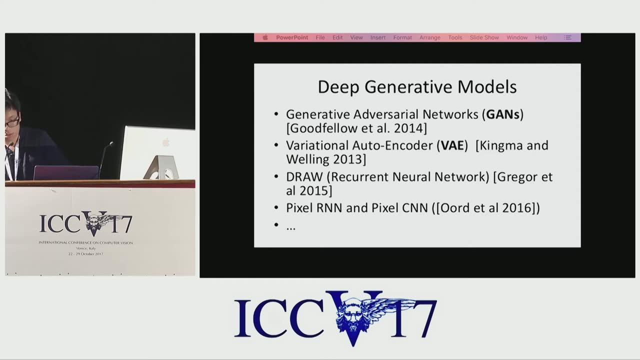 results. So my question is: rather than relying on the handcraft engineering, is it possible to learn a machine learning model to understand the real images and even create them? So this was made possible with the race recent development of deep generative model, So we will use GANs in this talk. This is among the best model and also 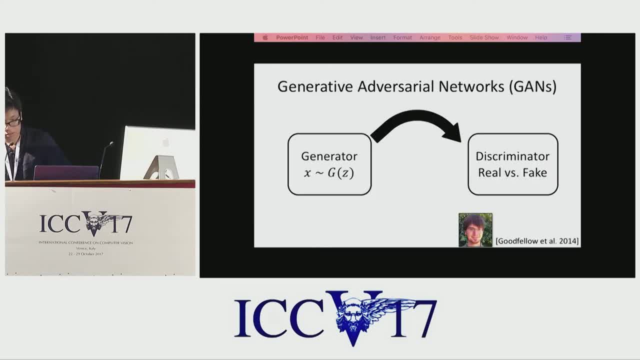 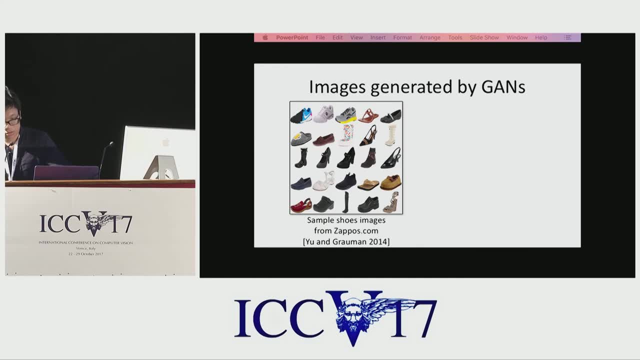 regarding the samples quality. So I will skip the GAN or will might repeat this too many times. So I downloaded 50,000 images from samplescom. I train a model with DC GAN code and actually the image quality are pretty good And but also, more interestingly, I, if you sample two random vectors and 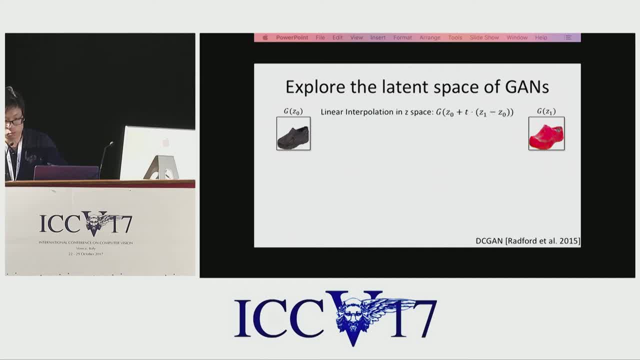 compute a simple linear interpretation between two random vectors, you can get a very smooth and meaningful transition. So I train a model on handbags I stole from Amazon and again it produced a pretty nice interpretation. This is actually pretty nice because during the training we never optimized for that In the 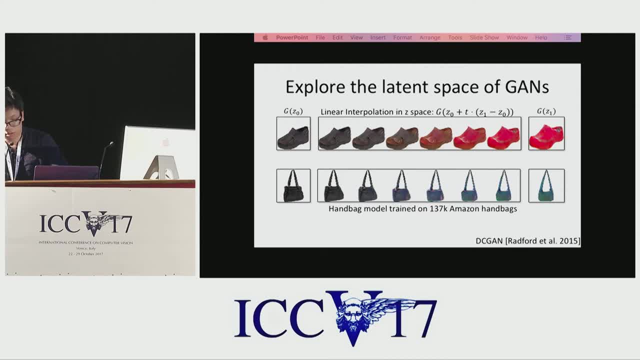 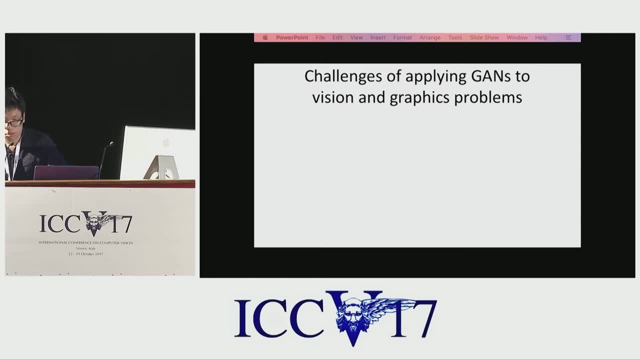 case, GAN might be a good model to model the image. natural image manifold So. but there are still big challenges of applying GANs to solving computer vision and graphics problem. First, it only allows you to produce a random images, And so each time it's quite hard to control. so if you would like to generate a particular image, there's no way to tell the algorithm. 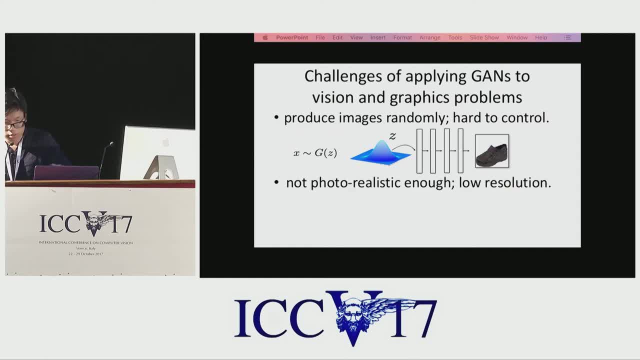 Secondly, the resolution is still quite low, like usually 64 by 64. So here if you look at images a bit lower, the result is fun. If you zoom in a little bit and zoom you further, the safety noals then look very real. So we will try to solve this problem one by one, and here we first present interactive tools to control the image. 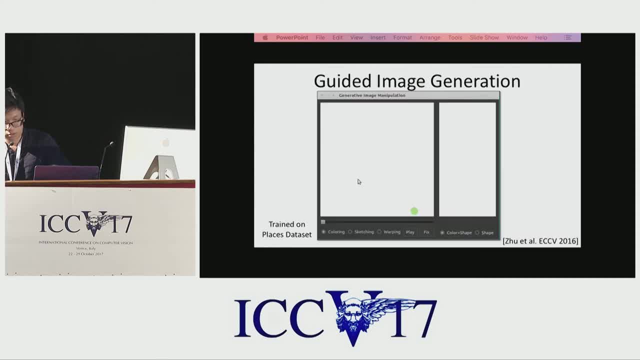 Let's run the program in the future version. You can also draw field scribbles and it can create an image which corresponds to the user's intent. So I want grassland with some brimstone, and here are different samples. I want to draw a mountain with just a triangle shape. 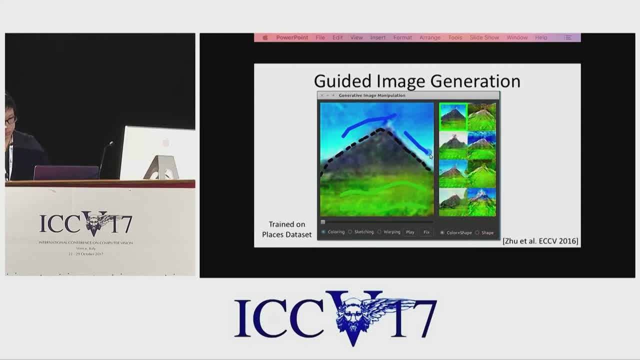 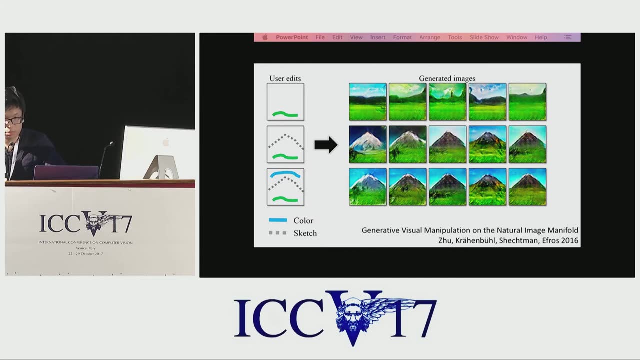 Maybe. I want a blue sky, I want to go skiing and we will have snowy mountain. So here, what we essentially do is we try to generate an image according to a user's edits. As a user draw edits more and more, and we'll create images accordingly. 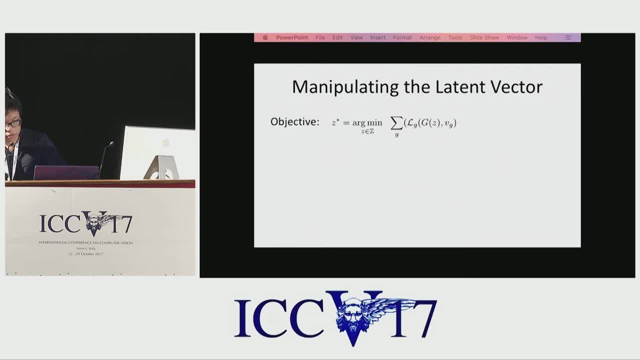 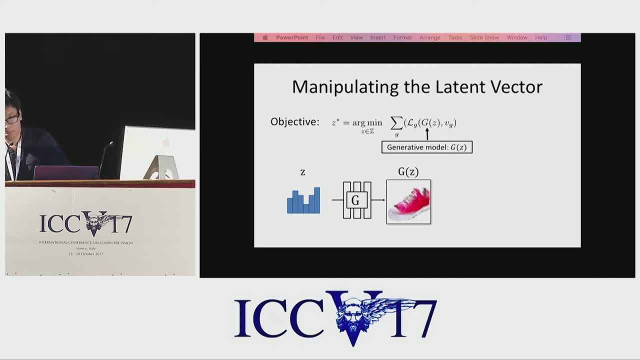 It's fixed. during this optimization We try to find the best random vector z so that it satisfies user's constraint. For example, here user draw a black stroke, want to make it show black And we can compute the loss function on this particular region. 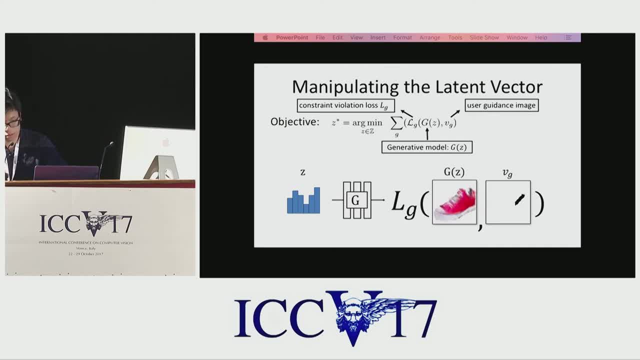 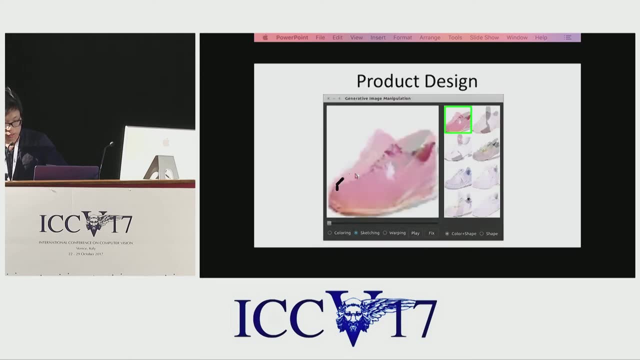 and just a very simple L2 loss in the pixel space And we can change the z vector so that it satisfies this constraint. And here are more examples: as user draw more and more strokes, It makes different parts of the shoes black. And let's look at example on shoes. 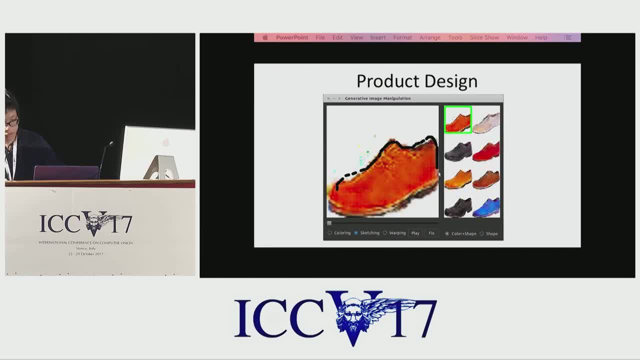 Here is a constraint on the shape and we can create different shoes with the same shape but with different color and texture And we can add more and more constraints. like I want the red shoes with a white button And I can add more. switch to the sketching tool which enforce the shape constraints. 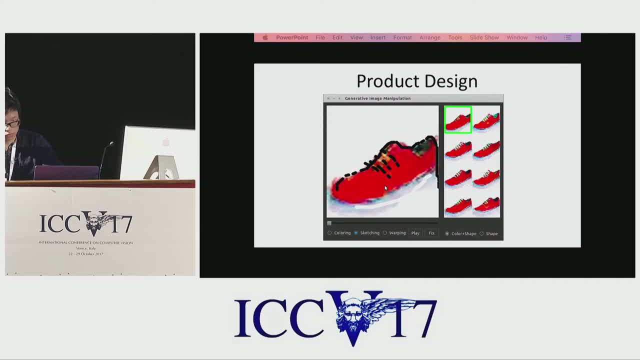 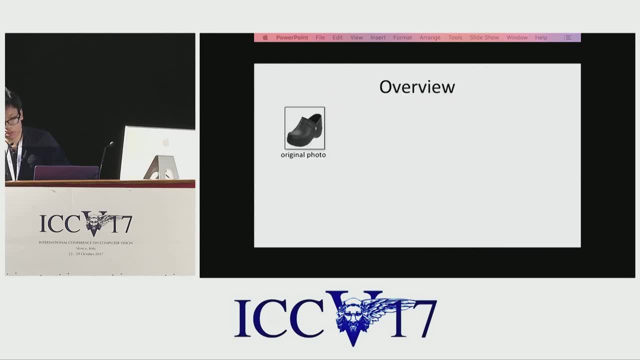 which we implement in a hog descriptor, a differentiable hog descriptor, And so it can add more details. So we can also use this tool to edit existing photos. So here is original photo We try to reconstruct using GANs And then we can have these tools as it's presented and generate different kind. 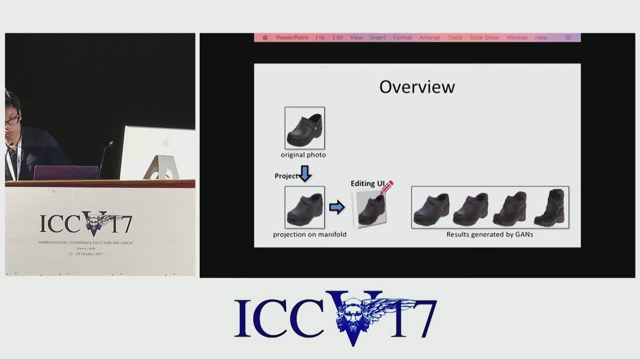 of output results. But question comes. so we start from a very high resolution image and end up with a low resolution results generated by GANs. So to generate final results, we basically what we did is we paste high resolution texture to the final GANs results. 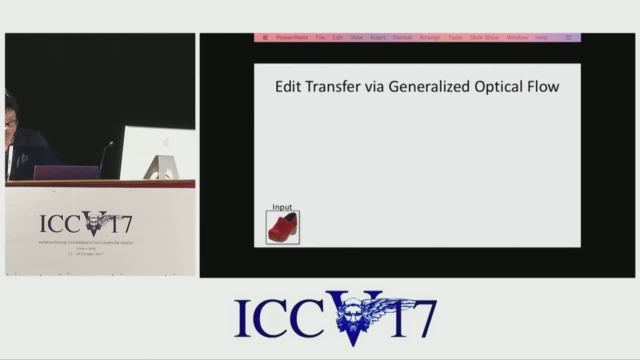 So let's go back to some very old topic: optical flow. So we have an import image and we reconstruct using GANs And we have final results generated by the editing tools. So how can we go from, given these three images, produce the final results? 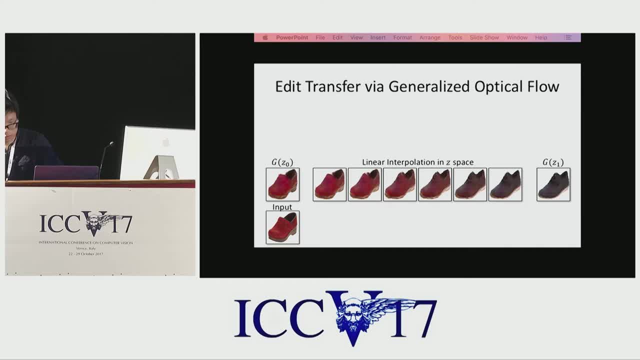 So again I show you some interpretation between the two random vectors. This is quite useful here We can actually estimate the flow. It's a generalized optical flow which can handle colors variation. So estimate the flow and apply the flow to the import images. 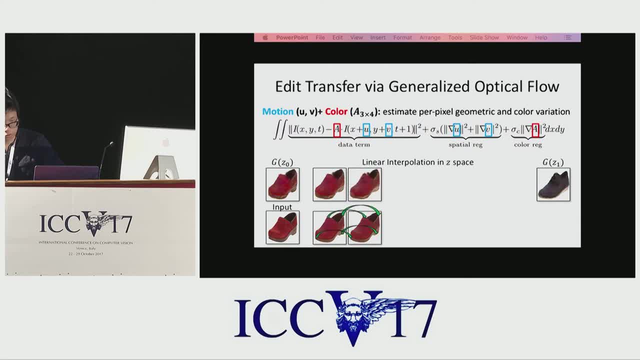 And we estimate the flow again between the nearby labels and apply the flow to the import real images And based on the change in the latent space we can apply the same amount change to the real import images. So here is a demo on editing the handbags. 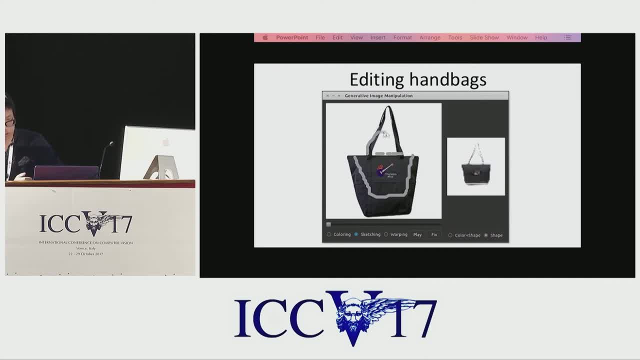 We draw a sketch And the right window shows the result generated by the GANs. It's updated real time And we apply the same amount of geometric change from the GAN space to the real image space. Here another example: We make a show a little bit thinner. 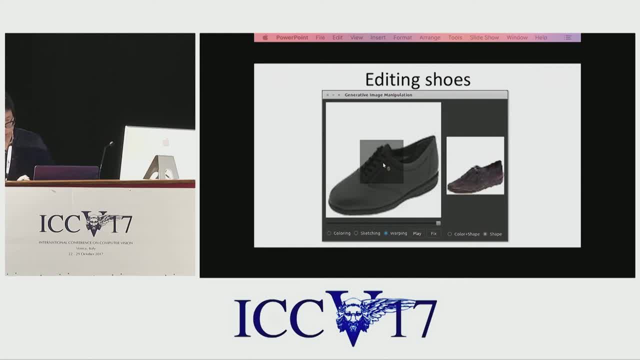 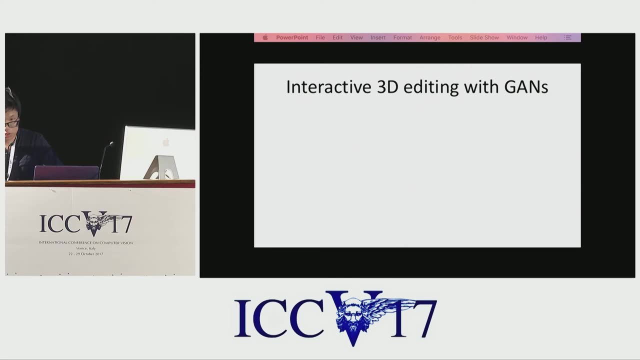 And we create results with GAN in the small window And we apply the same amount of geometric change with optical flow to the real import images. And there are actually some work. we're trying to apply the same idea into 3D modeling. So here is a paper from MIT. 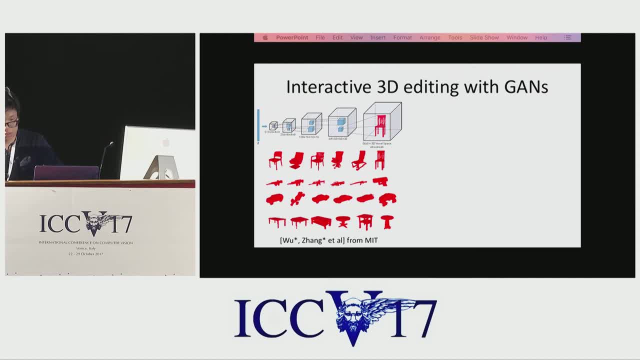 We try to synthesize 3D shapes with GANs, And here are the paper from Princeton which try to apply the same idea to control the latent vector to design the new chairs. Hello, OK, it's back. Thanks, And so we're going to go ahead and start the demo. 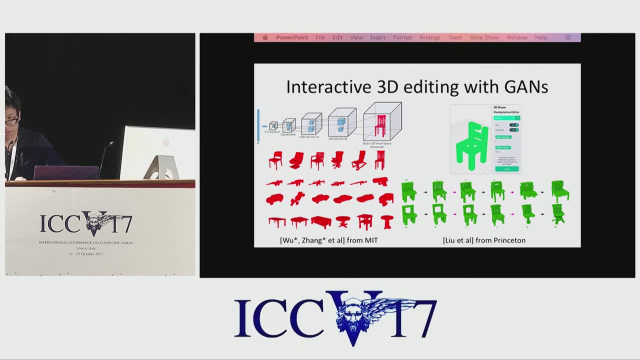 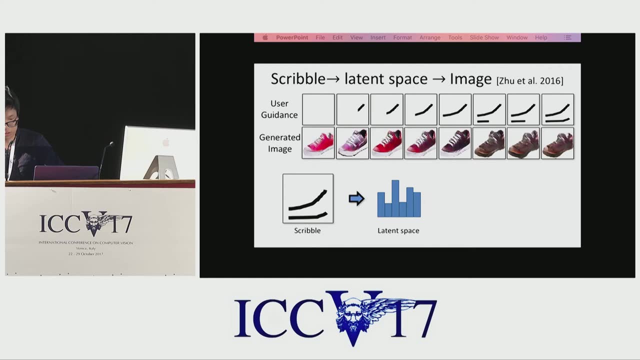 So, applying the same idea, they try to have a user interface to control the generation of 3D shapes. This is quite useful in 3D modeling and design industry, And so the idea of this paper from ECCV is we go from a scribble to a random vector. 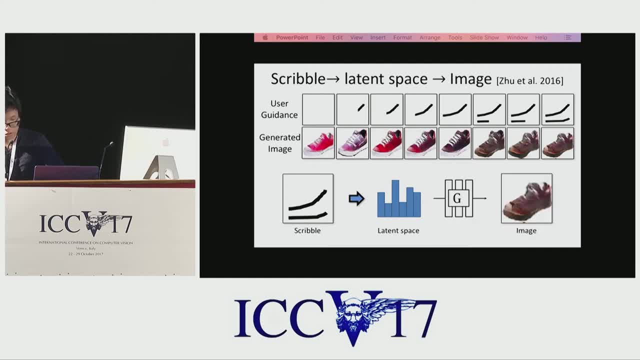 And then we use the GAN. We have trained to generate images And the GAN is pre-trained And we have some hand-coded optimization- either it's L2 per pixel Or it's L2 in the hog space- to enforce different kind of constraints. 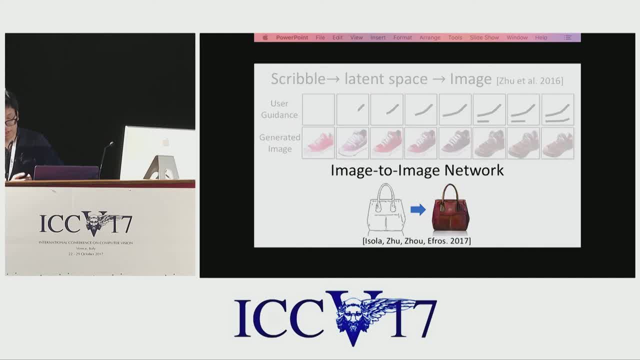 But in the end, what we would like to have is just a network to map the input sketch to an output, a handbag. We don't need all this random vector and latent space So we can apply the same idea out of a 3D loss. 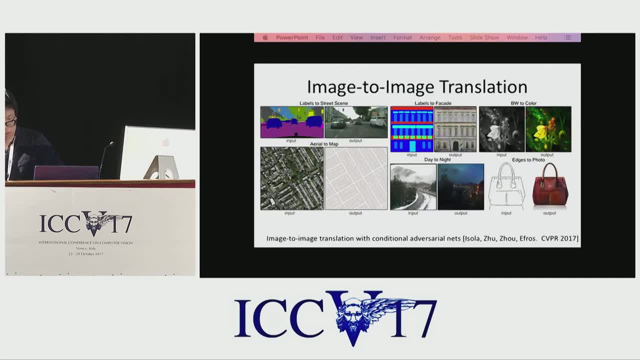 to solve this problem. So we propose an image-to-image translation, called pick-to-pick, for doing that. So this pick-to-pick allows different kind of application And we can do that with the same code base and same parameters. So is the leading author of this paper. 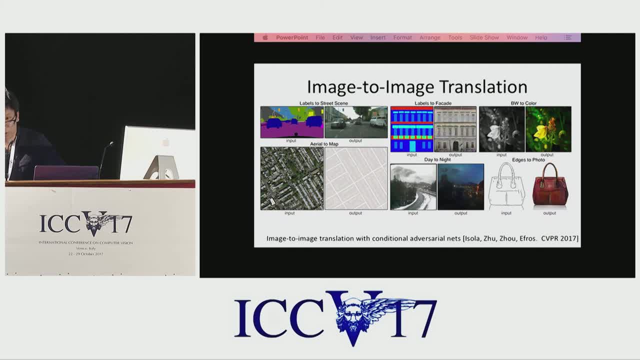 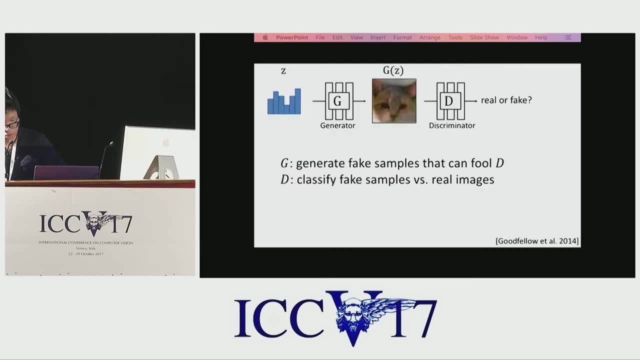 and who will join MIT next year. So many of the slides are borrowed from his job talk, So it's probably not bad. So let's look at the sketch to photo as an example. This is a regular GAN. We try to train a cat from a random vector. 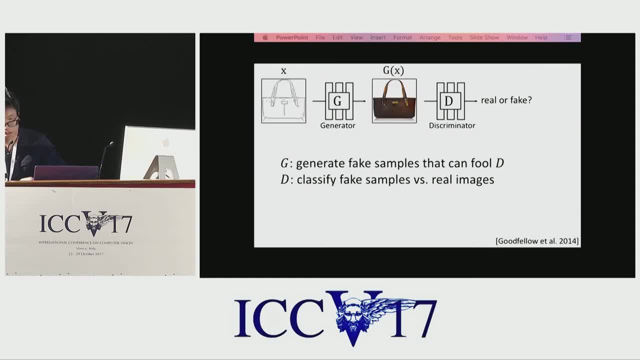 And here we just replace the input by the user sketch, by the edge map, and replace the output by the handbags. And but there is one problem. So there's only one issue. It's: this handbag looks real according to the discriminator. 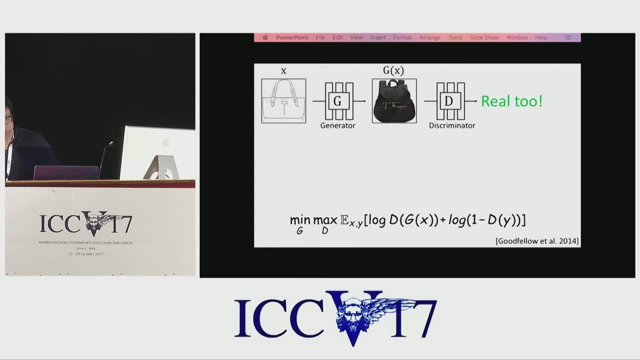 But this handbag looks real too. So the GAN doesn't enforce. the output correspond to the input. To address this problem, we add both the input and output to the discriminator. So the discriminator's goal is to classify if it's a real pair or if it's a fake pair. 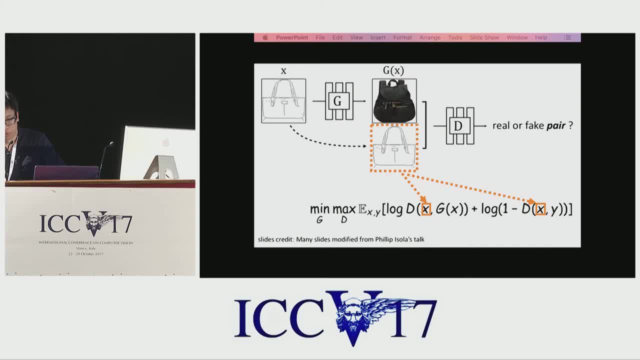 So we'll make it a lot more conditional, GAN, conditional on the input images. And now it just needs to say: this is a real pair And this is generated by the network. This is a fake pair. And then this is a ground truth: input and output pair. 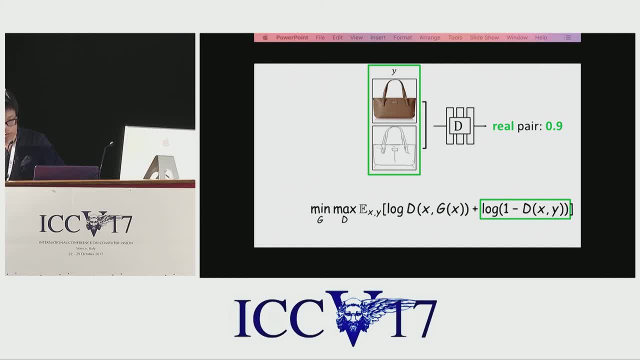 So it's real. So we just add this conditional variable to the networks And there are field training details to figure out. Usually it only involves three things: Objective, generator and discriminator. So let's talk about one by one. So for the objective, we found often adding a small L1 loss. 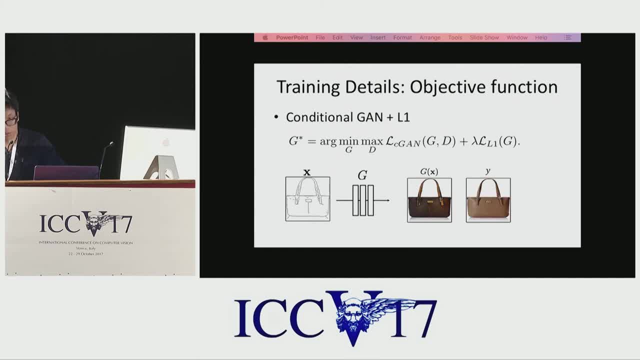 might help stabilize the GAN training. So L1 is more like a regression loss. So in pixel space we will try to predict the output and measure the difference between output and ground truth. And this always helps training GAN to stabilize GAN training. 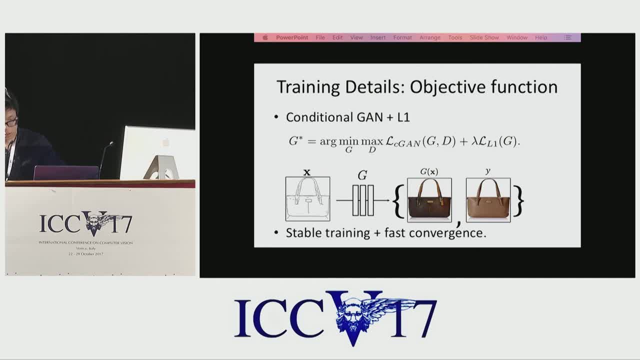 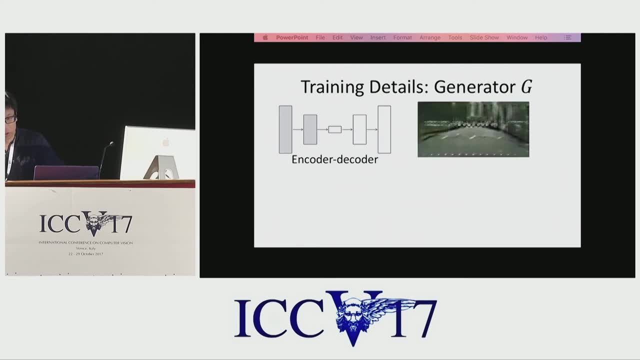 and makes everything converge pretty nicely. And also we have a different generator- always matter. So we try to encode the code architecture. You have a few downsample layer, upsample layers. It's produced pretty better results. But if we adopt the unit which is used for medical imaging, 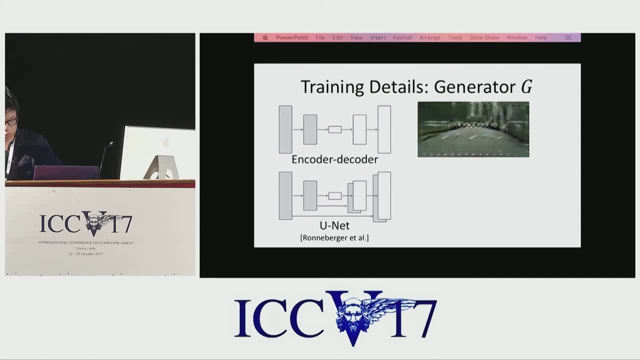 which connects lots of skip connections between the first layer, last layer, between the first field and last layer. it makes results much better. So even within the same adversarial loss, if you have different architecture, it actually matters a lot. So recently people are using ResNet or DensNet for that. 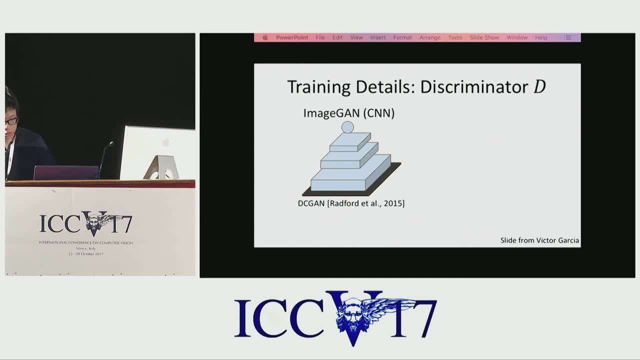 And also the discriminator also matters. So this is the convolution network used in DC GAN paper. What we use here is we call it patch GAN, which are trying to classify each 70 by 70 patch as real or fake, And it's a fully convolution network. 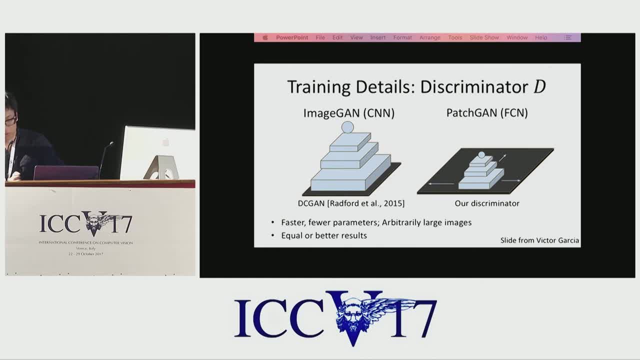 So you can run it across the entire image and it will tell you which patch is real and fake. This here actually has fewer parameters and produced the same or better results. This is because, in a conditional pick-to-pick case, the global structure of the output images 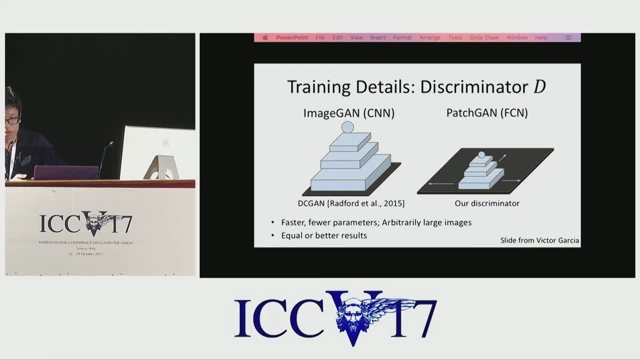 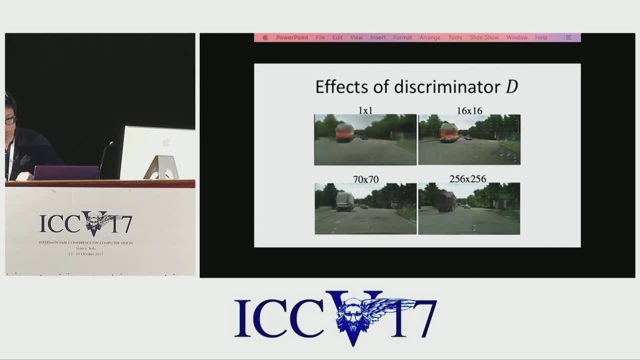 has been enforced by the input images, So they only need to care about if the local texture or local patch is real or fake. And here we see the same example. This is the patch size of the discriminator, Actually even the one by one, just 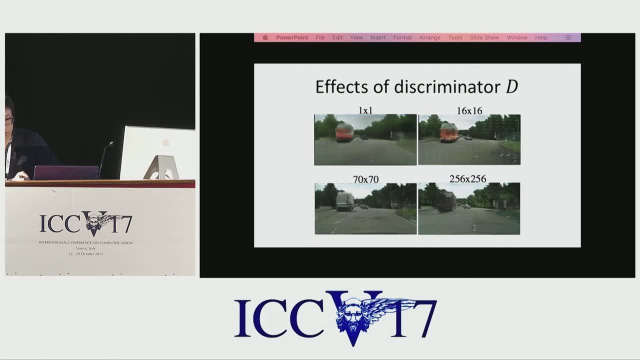 to look at this one each pixel and ask if the pixel is fake or real. This can actually match the current histogram of the results. So we found the 70 by 70 actually works at least as good as the full image discriminator, but it's much better, easier to train. 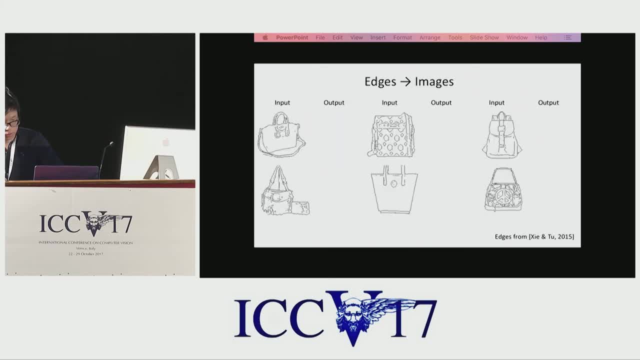 And here let's look at some results. So we adopted a model from EdgeMap to the handbags. These are some results we get, And note that it can not only hallucinate the color but also the texture at the bottom left case. 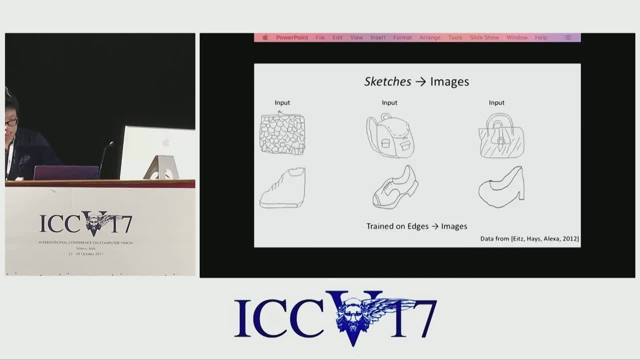 And also we adopted the same kind of code between from EdgeMap to the photo, but we adopted a user sketch collected by the Amazon Mechanic Turk, And here are some of the results we get. I see, of course the internet is not about handbags. 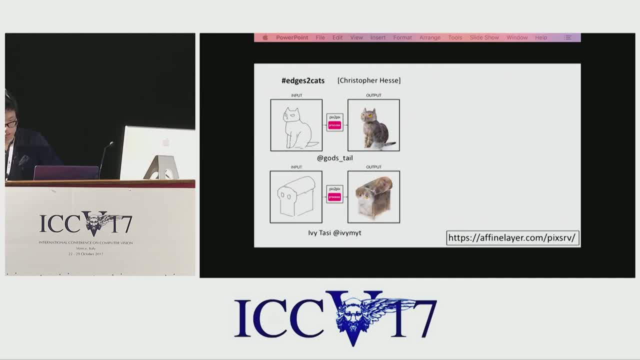 but about cats. We have already seen some results of it And here are more, And we are very thrilled for you to try the demo. Here are some more, And here are also some furry objects created by the artist. So the artist is very smart. 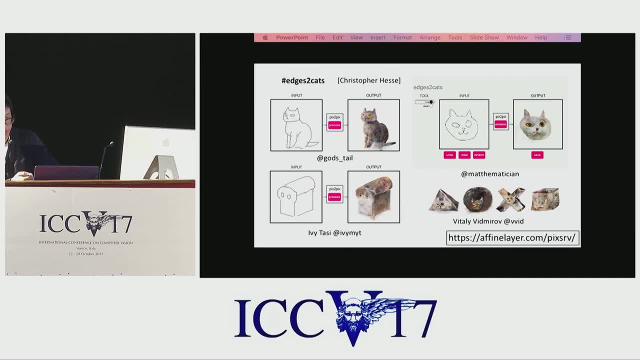 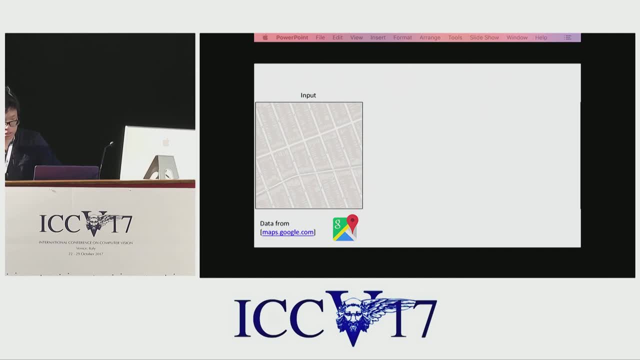 They don't show all the input So I don't know how to reproduce it. even I provided the code, So we can also pick to pick from other kinds of translation. Here is a Google And we can translate it into a satellite view. 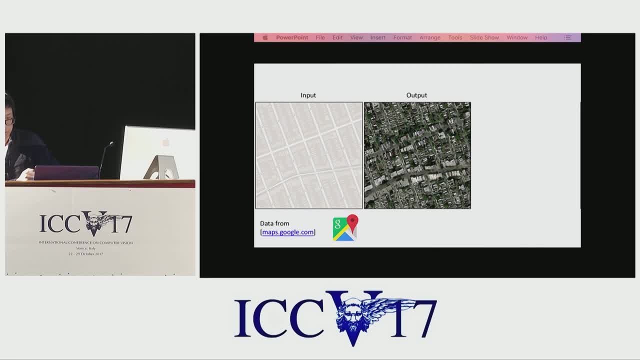 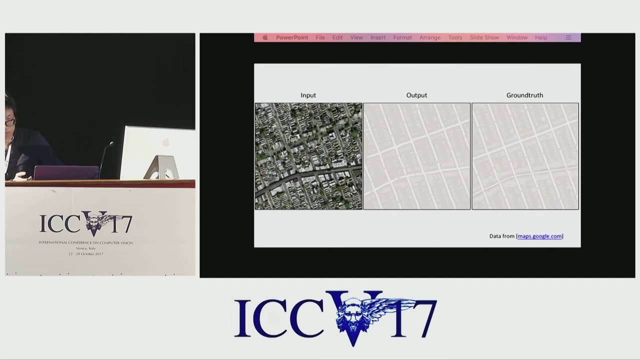 And this is actually a pretty high resolution. This is like 512 by 512. So it's very easy to generate. It's relatively easy to generate high resolution images in a conditional gain setting. And here are the ground truth images. You can perform the translation in the opposite direction. 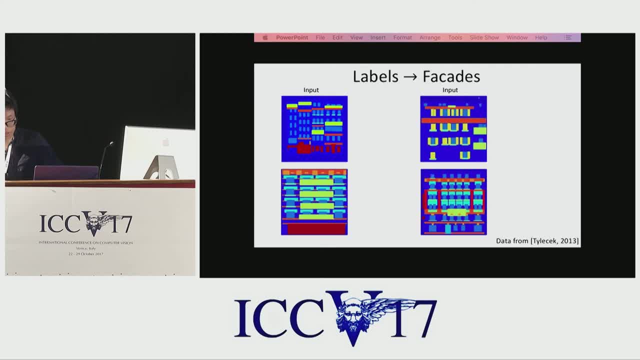 from satellite view to Google Map. And here are another application: We have the facade images, facade label map, which indicates if this is a window pixel or if this is a door pixel, And we can synthesize the facades based on the input. 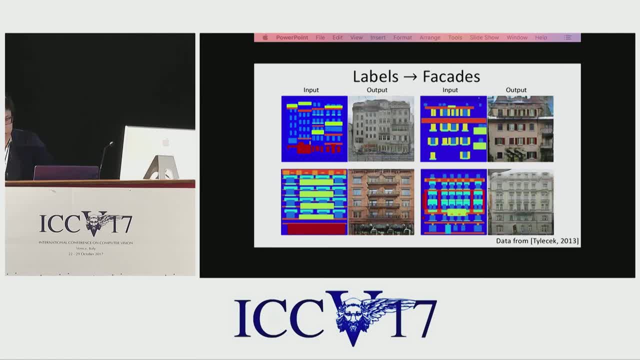 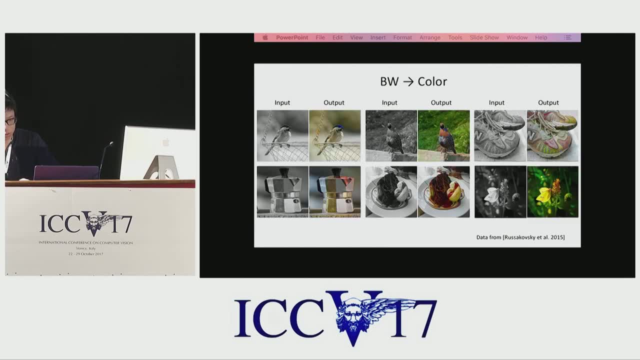 Again, you can add or remove some window and add or remove some doors, And it will change the results during real time. We also adopted the same idea to black and white images, to color versioning, And this can actually make the results quite colorful. 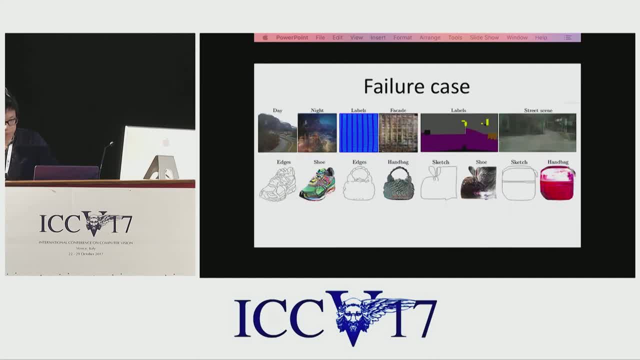 compared to L2 regression loss. Of course, the method will fail And sometimes if the input looks like a very unusual or very new, it doesn't work very well. Or if your sketch is very bad, it doesn't work very well. 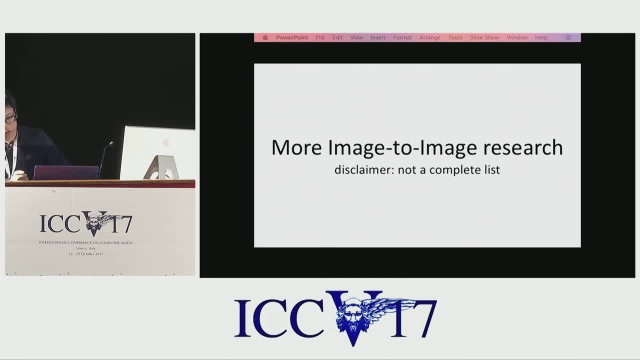 So we are not there. There are also many, many people in computer vision and the graphics community are starting using conditional gains to solve image-to-image problems. So here I will give a few examples, But there are around hundreds of papers. I didn't intend to give a complete list. 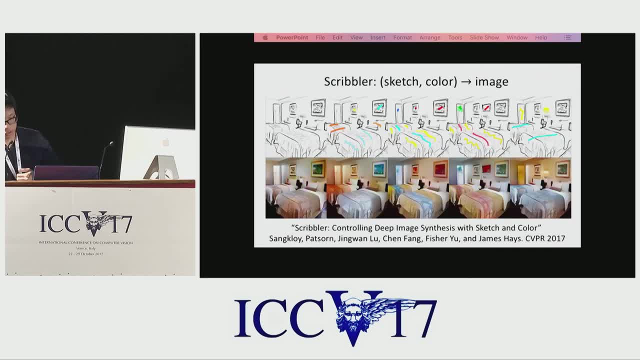 So here the first project is scribble from Adobe and Georgia Tech. So they tried to generate new images based on both the user sketch and the color sketch, so that the user has more control of which kind of images he would like to produce. 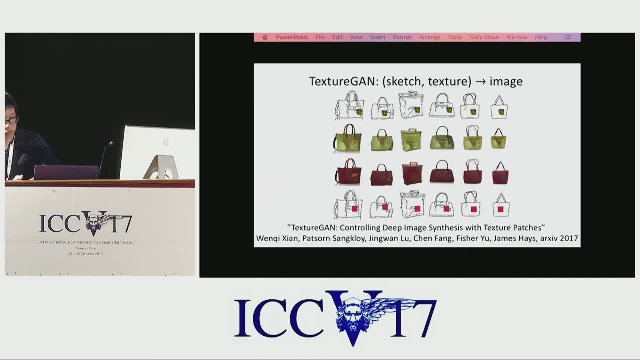 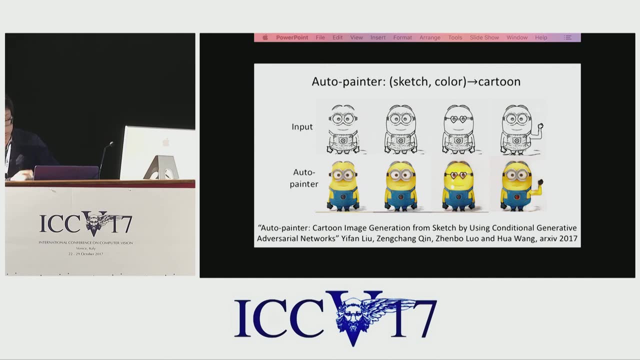 And also from the same group. they send this message to take both sketch and texture patch as input So you can select a texture from a dictionary and produce different kind of results. Again, I think image-to-image are also used in cartoon colorization. maybe have black and white. 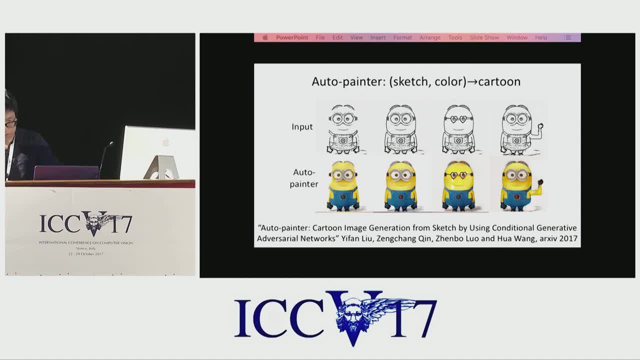 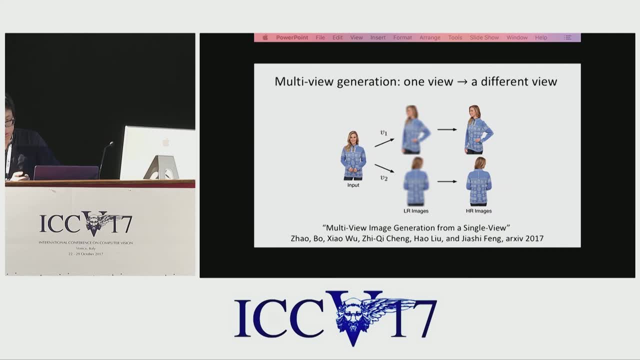 cartoon. You can colorize it automatically. Also, it's used for new view generation, view synthesis. whereas the goal is to give an input view, Your network tries to generate a different view of the same person or same object. Here they adopt a stack and message. 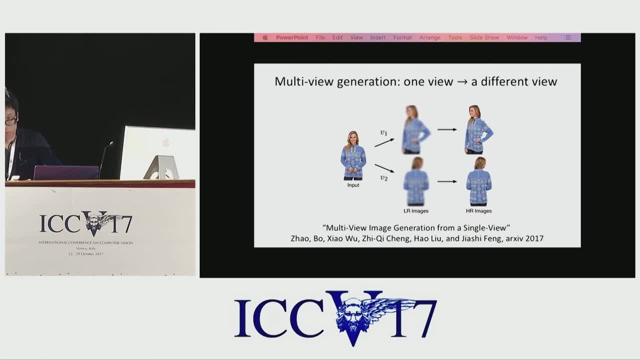 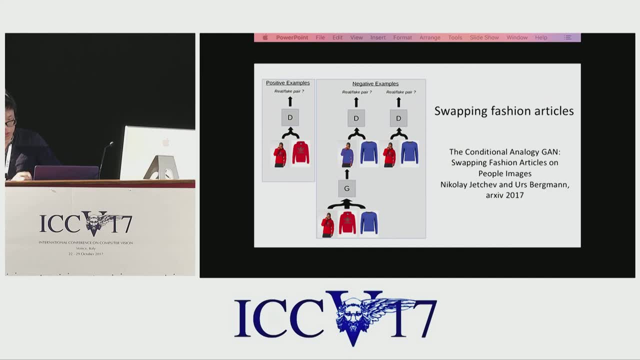 They first generate load of images and then have another network to produce details. Also, the image-to-image model can be used to generate new fashion articles with your own photos. It takes three images: a photo of a person and that particular fashion article. 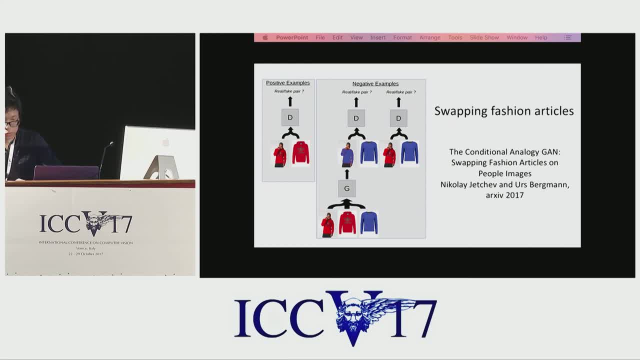 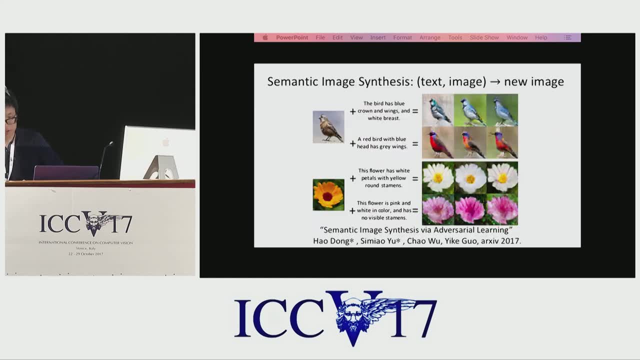 and a new fashion article, and it can generate new results, given a different fashion article. Image-to-image translation can also be combined with the text-to-image synthesis. Here we would like to synthesize a new image which looks like the input image, but also 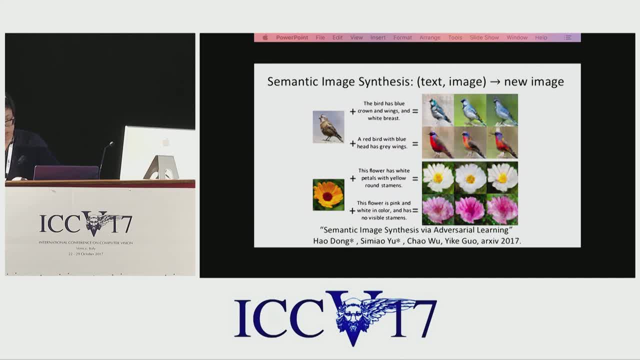 follow the description of the input text. For example, here the description is: the bird has blue, clone and wings and a white breast. So it will change the wings to blue and also the breast to white, but also looks like this: input image, post and identity. 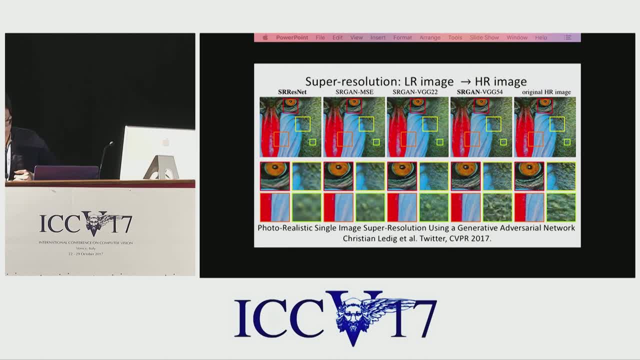 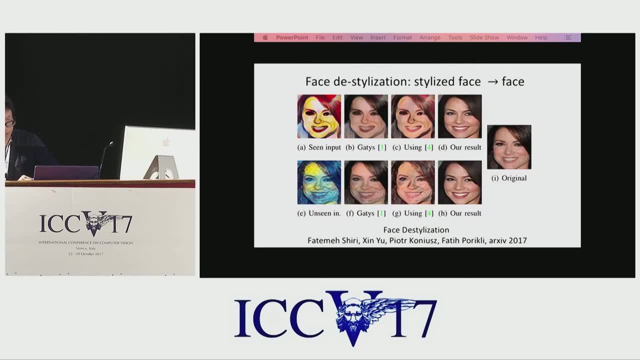 Of course, GANs can produce much sharper results for superlative solution applications Here. another interesting application is called face desterilization. It's basically we saw the style transfer results, but how could you get recovered original image from the style results? 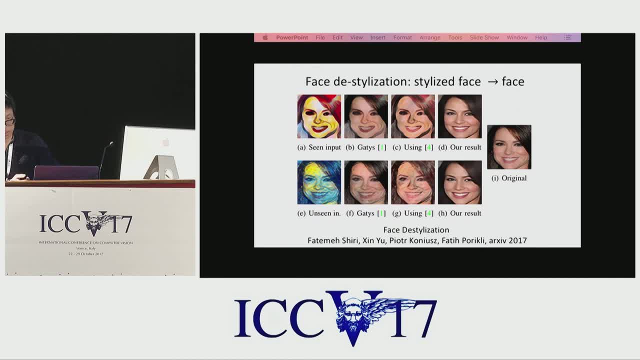 You can train out of a certain network to doing that. Also, it's very easy to get training data. You just apply the stylized algorithm and use the input, and your original image is output. You can train a conditional GAN model on using your training data. 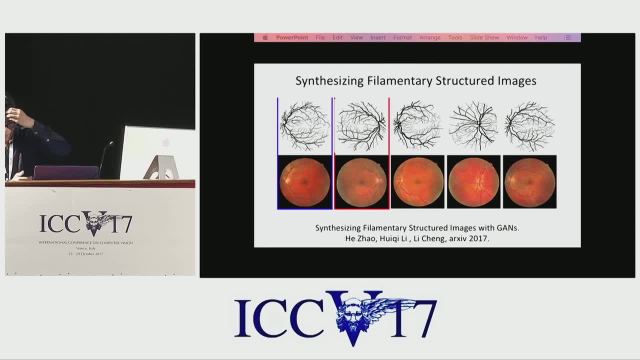 And also even in the medical imaging domain. we are seeing many, many, Many paper trying to generate different kind of imaging data from different kind of input domain. Here is the ground truth of the labeling. You can synthesize actually the image of eyes. 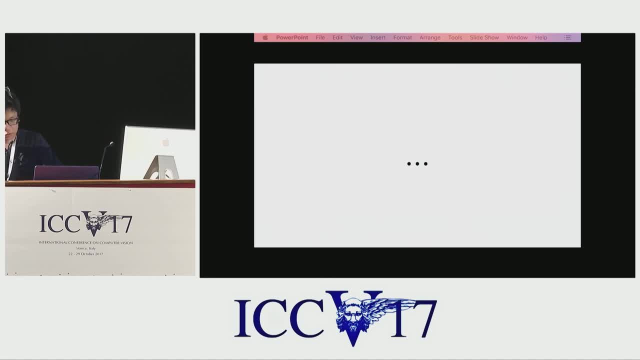 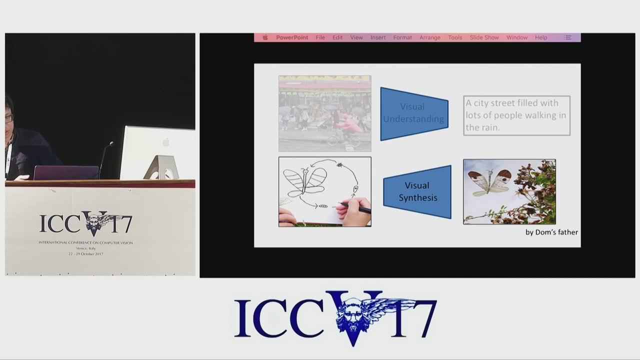 And there are many, many more applications. We urge the readers, the audience, to read these papers. So, in conclusion, we were inspired by this DOM stream. So our ultimate goal is to allow any people to create, you know, realistic images from some mental pictures. 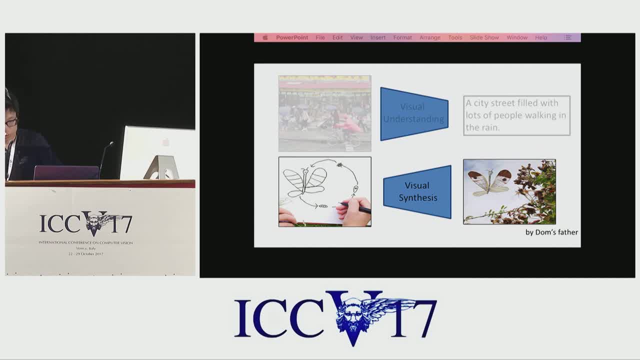 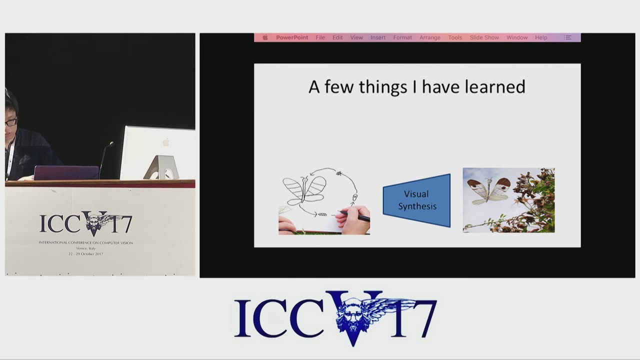 So there can be different kinds of user controls And we have done a few projects on that, from again to pick to pick, But still similar to the unconditional GAN. we need to further improve the quality and the resolution And also a few things I learned from my research is: 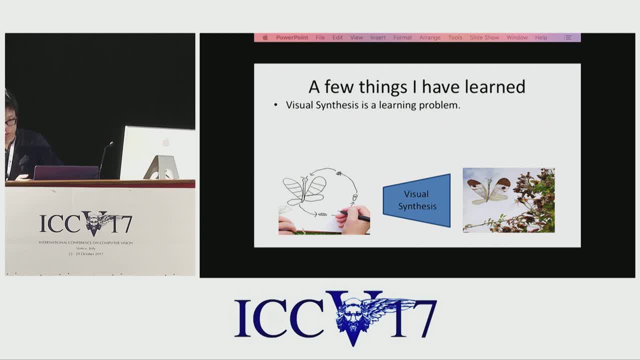 I think the image generation, vision synthesis, could always be modeled as a learning problem. Right, Yeah, Yeah, Yeah, Yeah, Yeah, Yeah, Yeah. And actually we can learn it. The supervision comes from children's photos. We don't need even to have an image net. 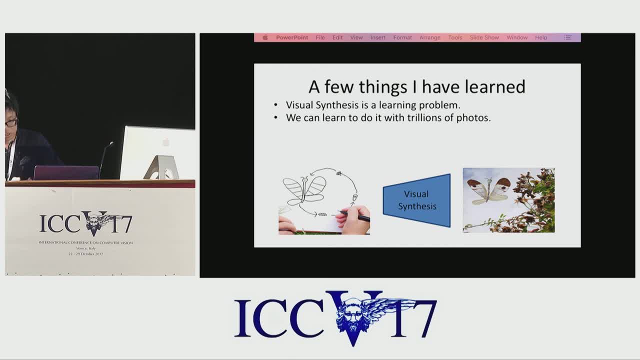 We don't need to even label a single image And we can. there are so many images we can learn from And also the conditional GANs, or image pick to pick kind of stuff, are much easier to train and often converts nicely. 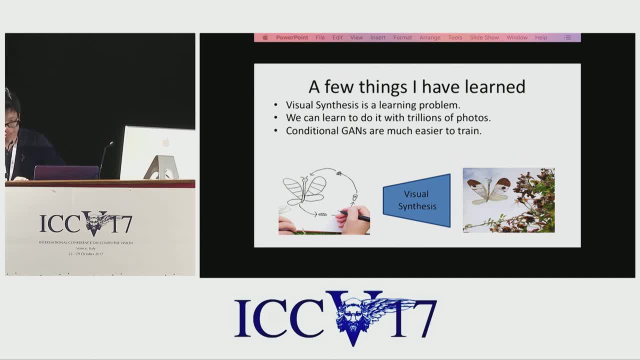 So if you are not smart enough to train unconditional GANs, you are very welcome to solve image to image problems, And it's also also also also very good to build general purpose tools which can work for multiple problems. 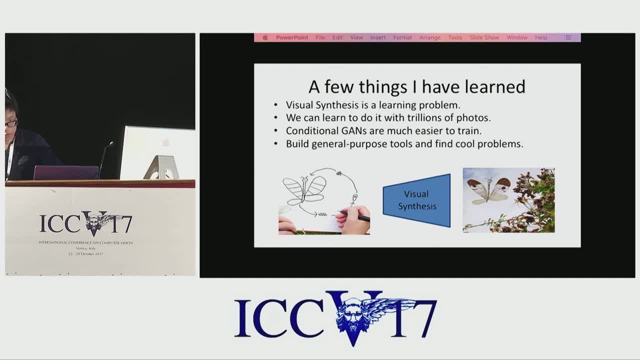 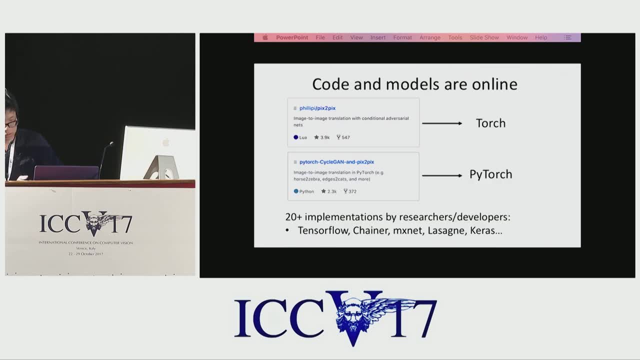 And like pick to pick framework is among these And we are also happy to open source the code. So we have both the Torch and the PyTorch version on GitHub And they are kind of very popular- thousands of stars- And they are also, more importantly, 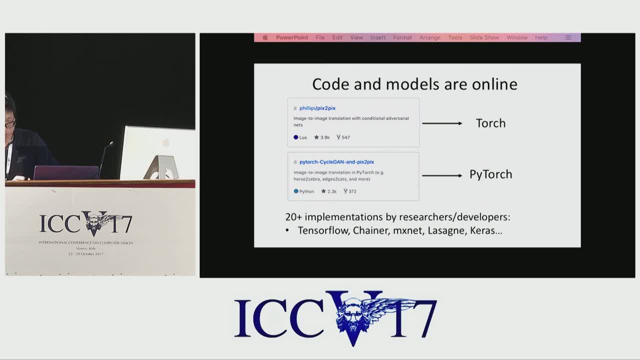 they are actually different implementations by researchers and developers. Even a TensorFlow version is actually very popular, like 3,000 stars, So actually they have different implementation. You are very encouraged to try it on your own masters, So the only thing you need is to have the input images. 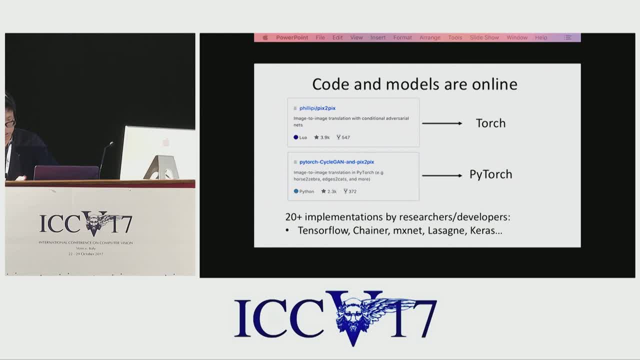 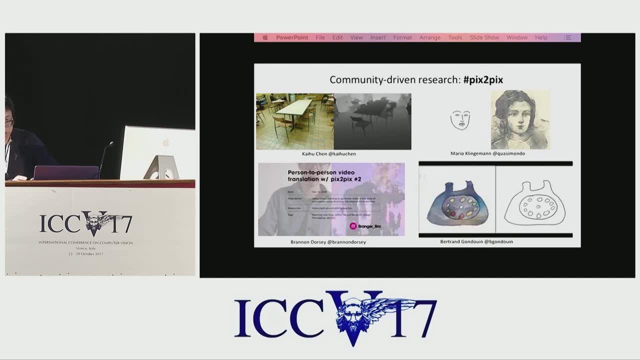 output images and it can produce the results for you without even reading the code, And I think- and I think Yang and Kong argue that maybe the archive versus the traditional publishing model, but I feel like the most recent results are actually from Twitter, not from archive.